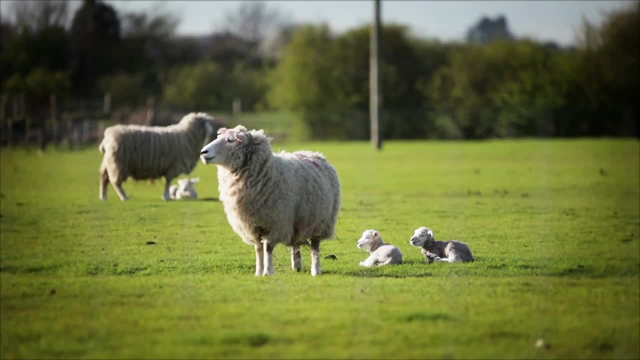 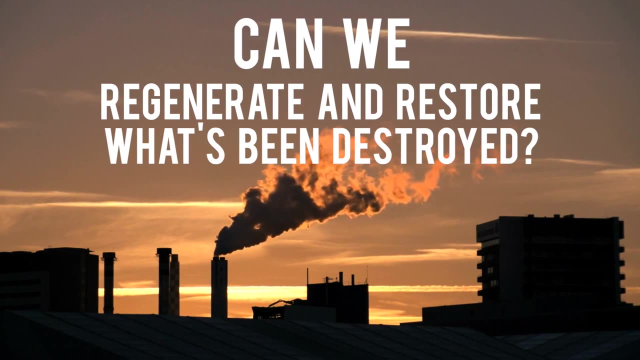 survive, a way to live on this planet in harmony with other life forms, a way to regenerate and restore everything that's been destroyed since the beginning of the Industrial Revolution. Is it possible to do all of this and to feed a rapidly growing population? 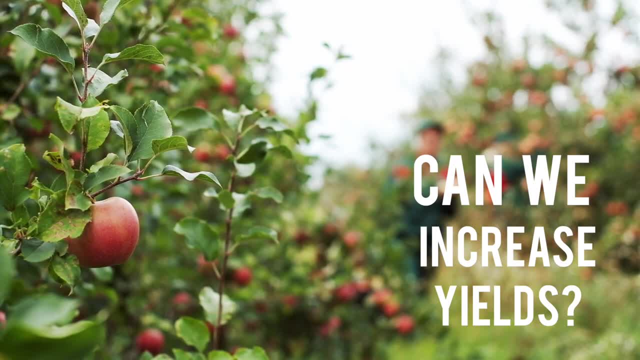 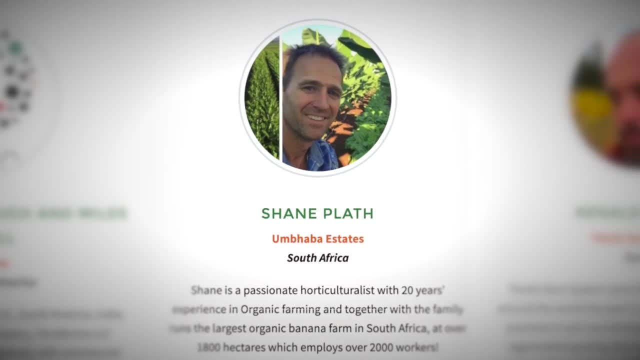 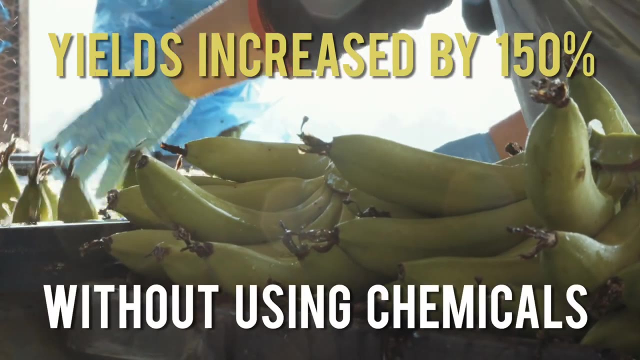 Is it possible to maintain or even to increase yields without the use of chemicals. Organic banana farmer Shane Plath farms 5,000 acres in South Africa. He discovered a way to increase his yields by 150% without the use of any harmful chemicals. How was he able to do this? The answer lies beneath the surface. 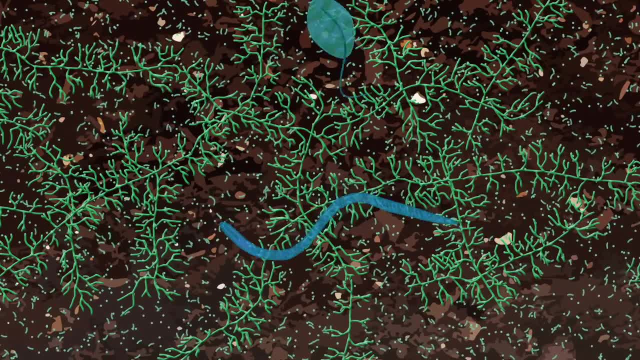 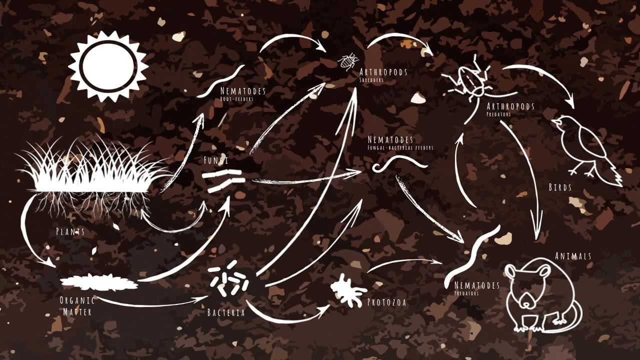 of the soil in the microbial community that dwells here, known as the soil food web. When left undisturbed, this diverse ecosystem is the perfect place for plants to thrive, and it's where plants first began to evolve. But the majority of these organisms can no. 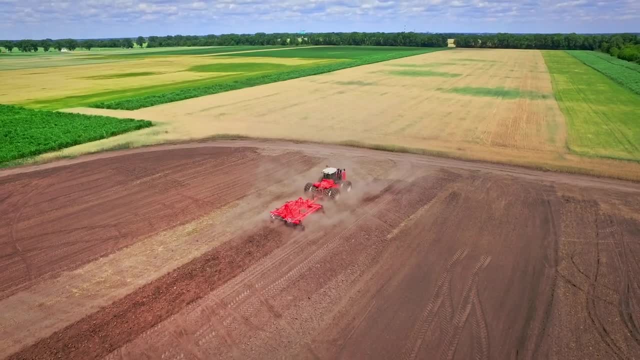 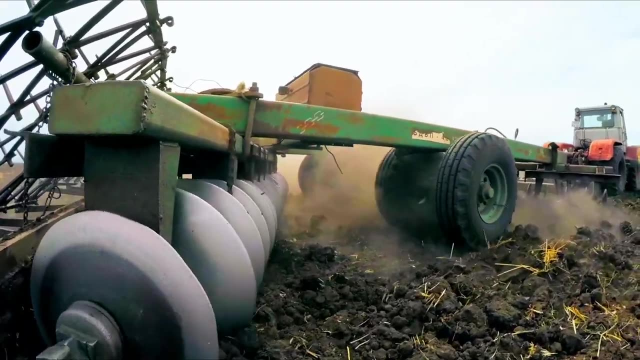 longer be found in agricultural soils, as the mechanical plow has destroyed many of the groups of larger organisms, such as beneficial fungi and nematodes. When farmers started using tractors to plow their fields, they unwittingly destroyed the ecosystem that was nurturing and protecting their plants. 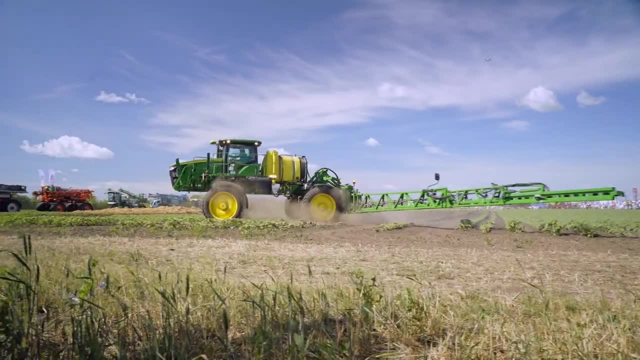 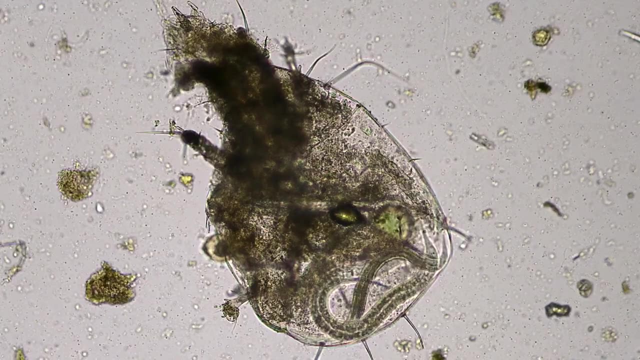 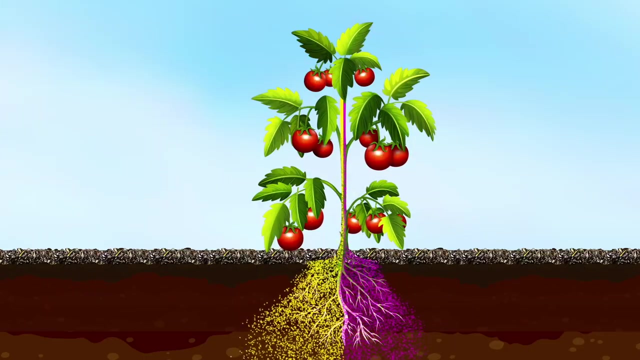 leaving them susceptible to disease. Then along came the toxic chemicals, which have resulted in more destruction. It's time to go back to nature's own operating system. It's time to restore the biology to our soils. Beneficial microorganisms provide plants with nutrients, which they harvest from. 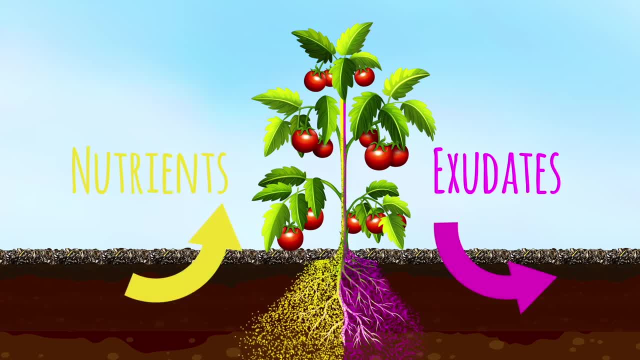 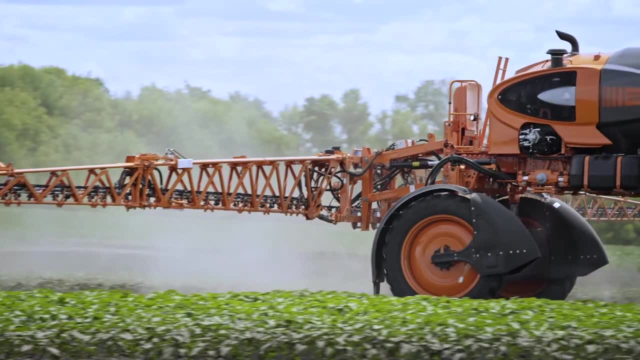 the soil, and they protect plants against diseases and pests. Surprisingly, the biology is also capable of mopping up the toxic chemicals that we've been putting into our soils. Some fungi have recently been discovered that can absorb crude oil and even plastic, which they view as foods. 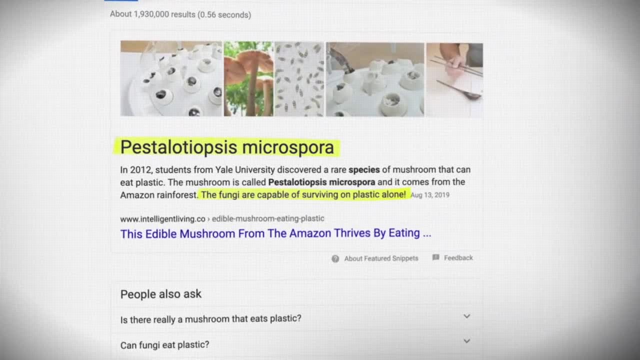 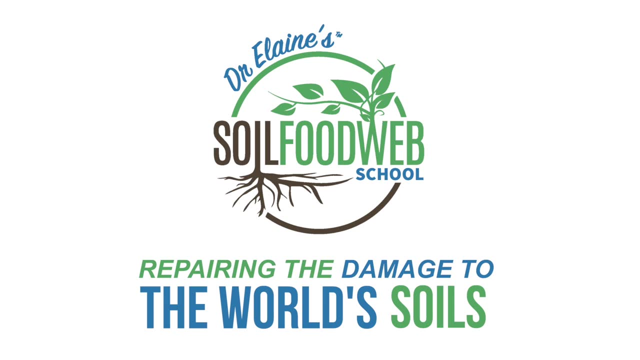 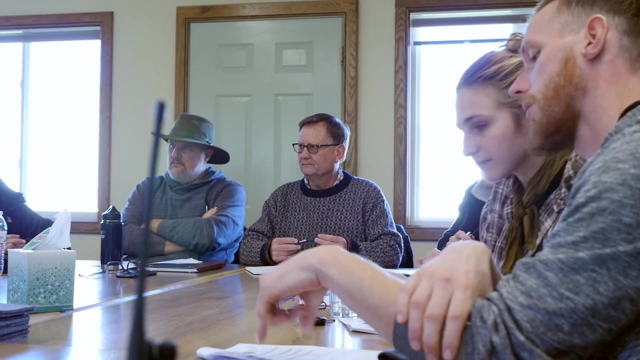 So the good news is that the damage we've done with chemicals can be repaired quite rapidly. This is our focus: repairing the damage to the world's soils. At the Soil Food Web School, our mission is to empower individuals and organizations to regenerate the soils in their communities. We train folks with 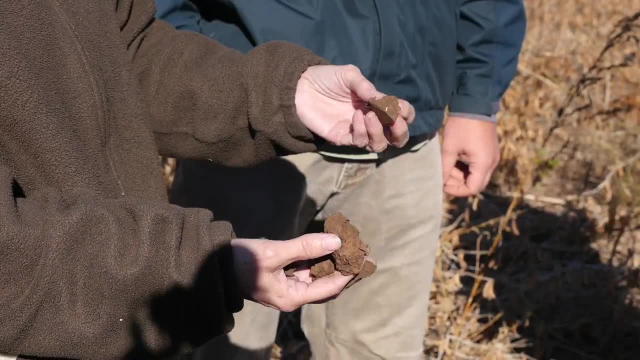 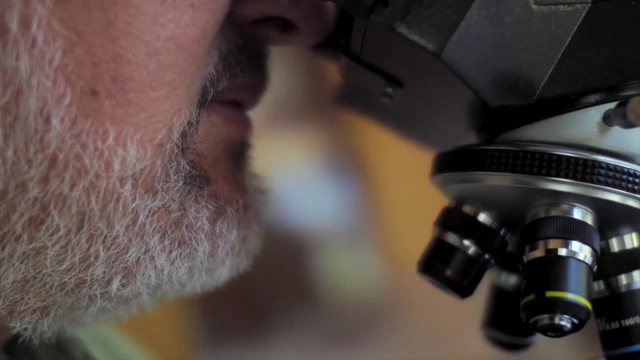 all sorts of different backgrounds, not just farmers and agricultural professionals. Many of our students don't have a background in agriculture at all, but are individuals who are really passionate about the planet And who are looking for a new career where they can make a big impact on how. 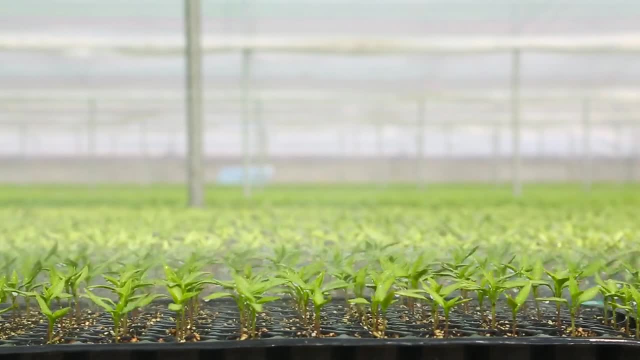 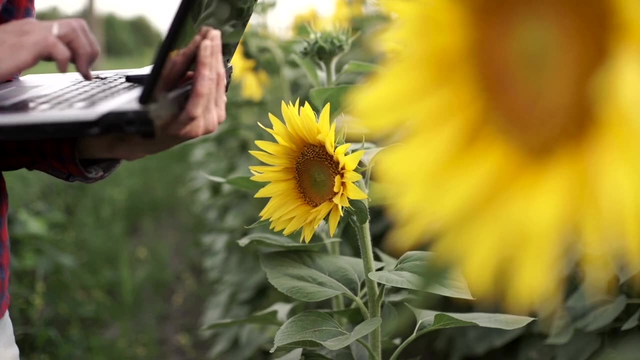 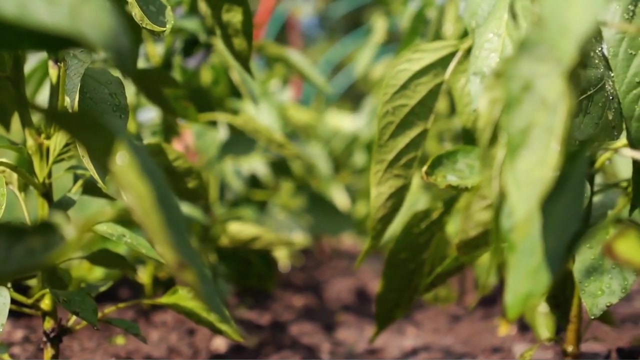 the soil and our waterways are being treated and on how the food we eat is being produced. Supporting farmers to make the transition away from using chemicals to a regenerative agricultural approach can be very rewarding. As a Soil Food Web Consultant, you'll be able to help farmers to accelerate their soil. 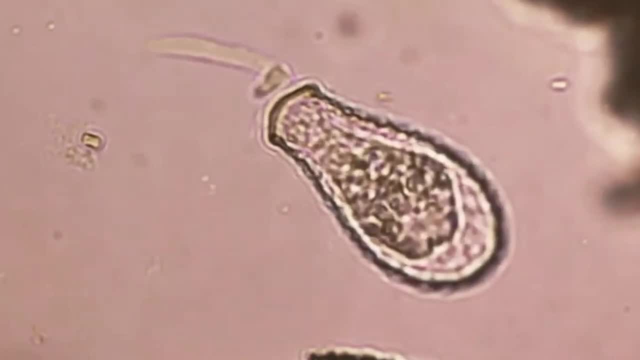 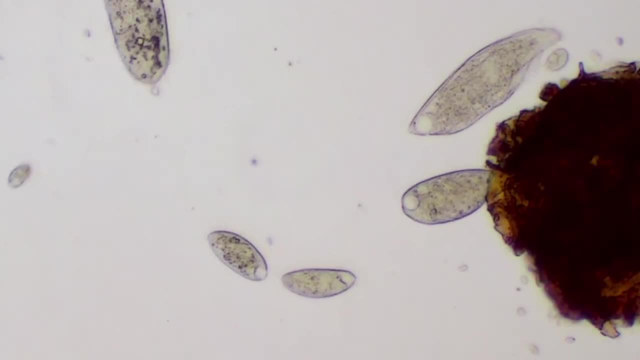 regeneration efforts by focusing on the soil microbial community that forms the foundation of a healthy soil. Soil food is one of the most important systems that drive the system. So by giving the soil biology a boost right at the beginning of a regeneration project, you can help your clients to see results in weeks or months. 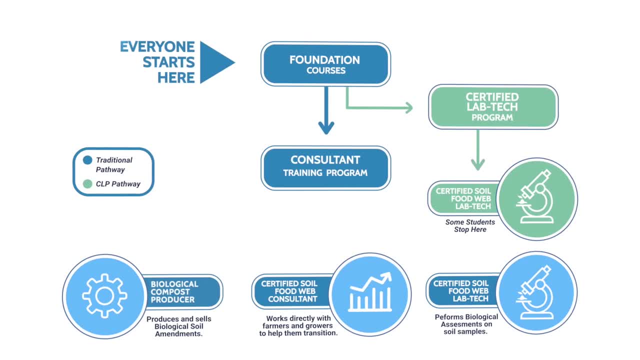 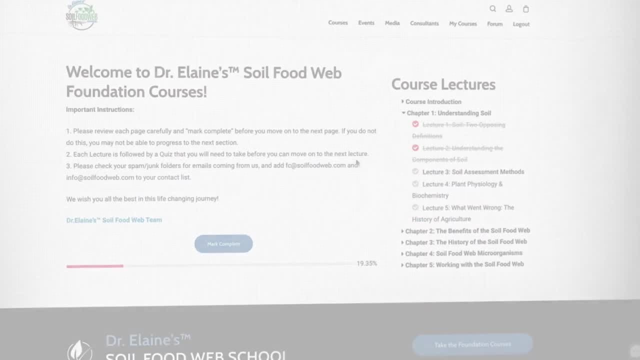 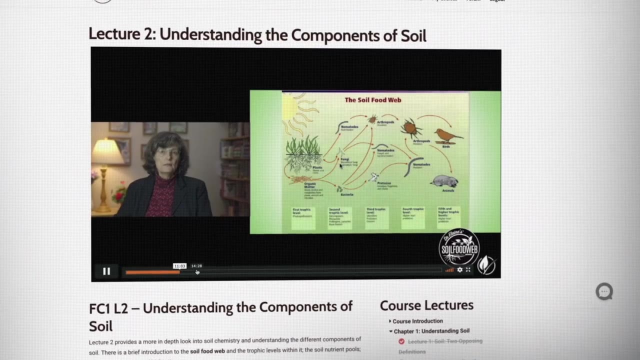 rather than years. Let's take a look at some of the training programs that we offer at the Soil Food Web School. Everyone starts here with Foundation Courses, where they cover all the science and application methods behind the Soil Food Web approach. This is a series of 63 self-paced online lectures, each followed by a quiz You can 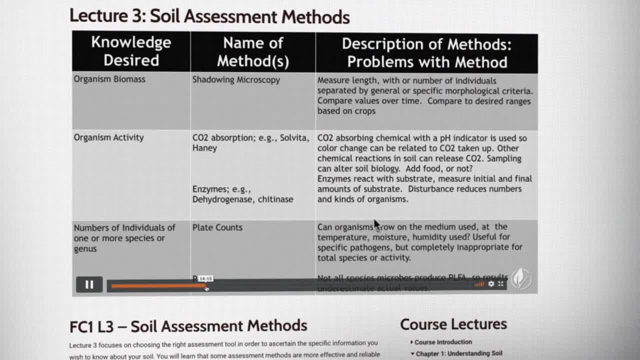 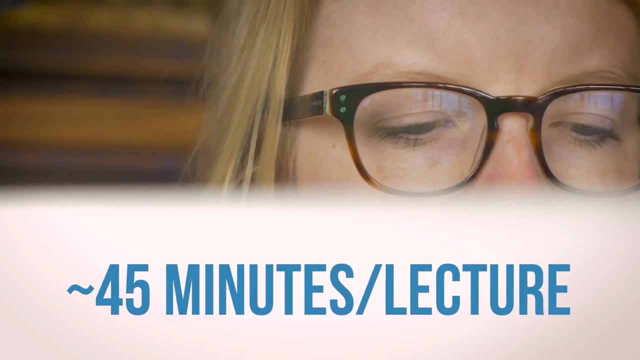 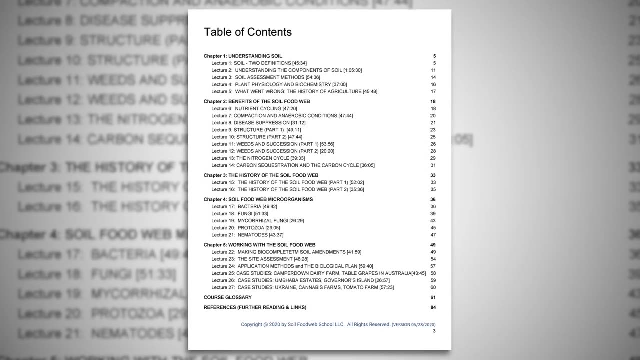 log in at any time, watch a lecture as many times as you'd like, prepare your notes and then take a multiple-choice quiz. Each lecture is approximately 45 minutes in length, and we recommend that you dedicate around 150 hours to completing the Foundation Courses. The lecture slides in the Foundation Course. 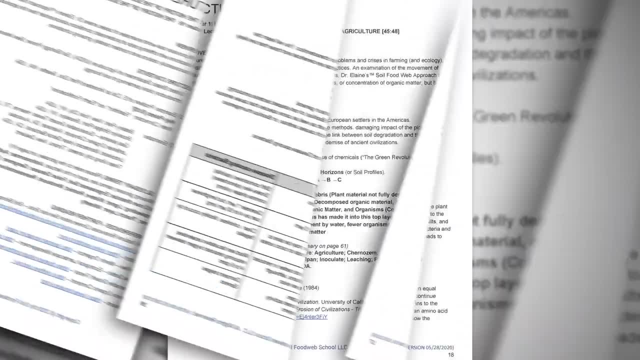 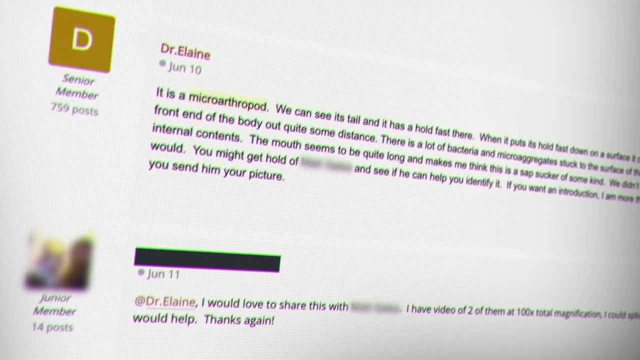 Manual are downloadable so you can create your own library of reference materials. During the courses, you'll have access to the FC Forum where you can ask questions that Dr Ingham and her team will answer for you. You can attend monthly Q&A webinars with Dr Ingham and other members of the faculty. 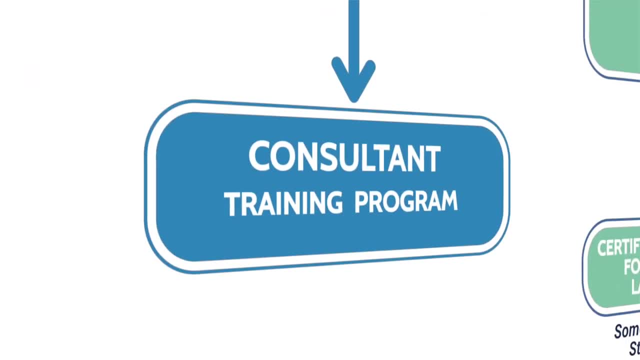 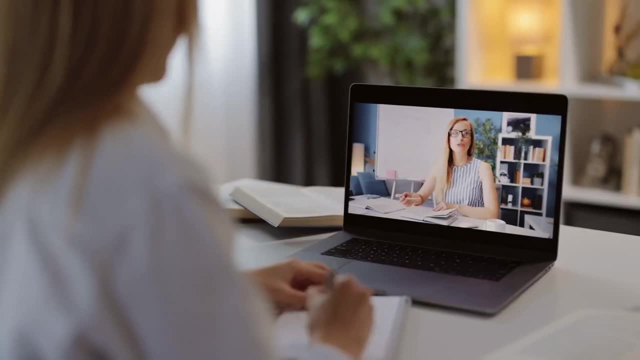 After you complete the Foundation Courses, you can then elect to move directly into the Consultant Training Program, which is where you'll put all the theory into practice with the guidance and support of one of our highly qualified mentors. Some are Soil Food Web consultants who run their own businesses supporting farmers to 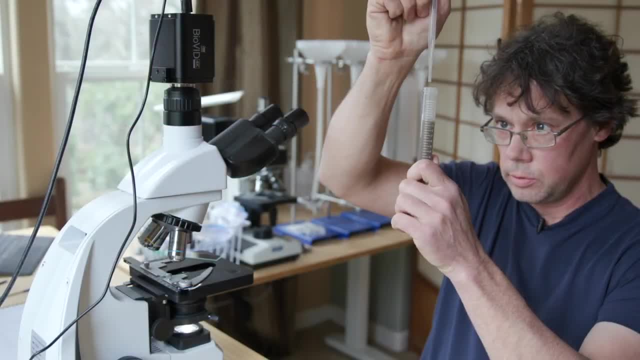 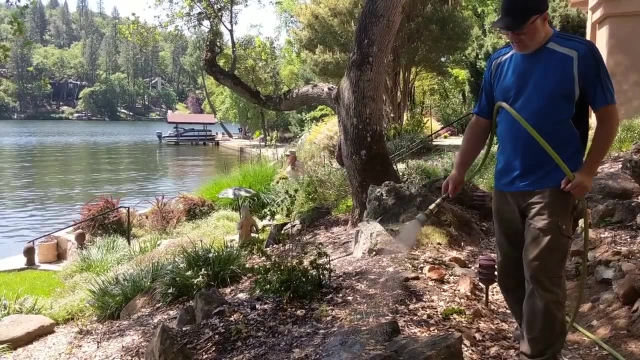 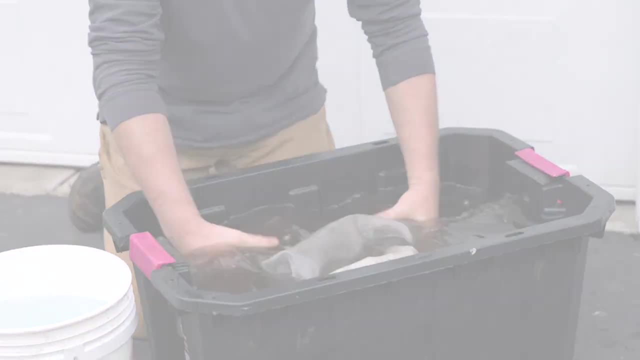 make the transition into the Soil Food Web approach, and others are PhD biologists who have been working closely with Dr Ingham for several years. Our mentors have worked with dozens of farmers in all different kinds of settings and they work together as a team, sharing experiences and solutions. 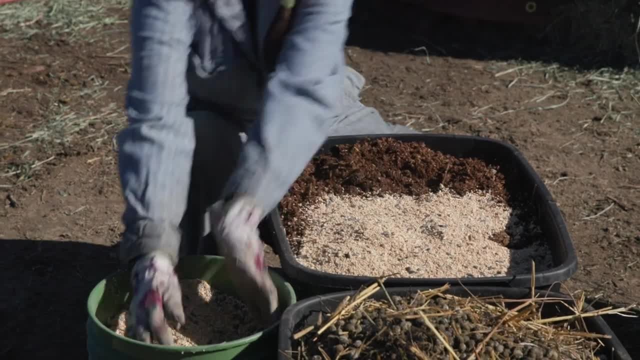 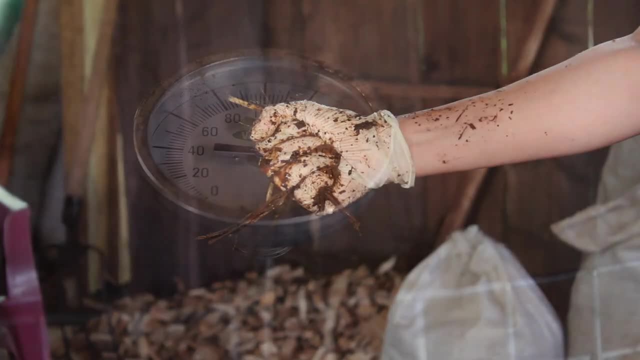 In Stage 1 of the Consultant Training Program, you will be challenged to make Biological Compost. Your mentor will support you with the guidance on how to avoid making common mistakes and how to tackle some of these challenges that are unique to your situation. 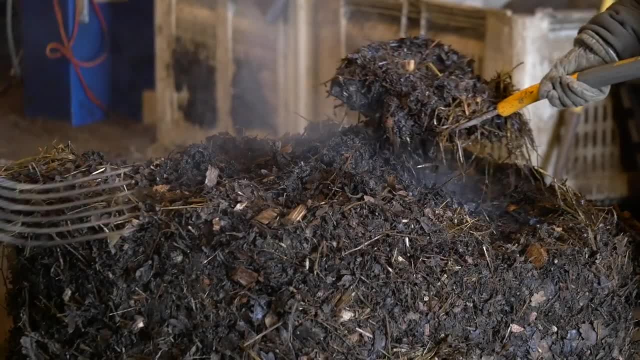 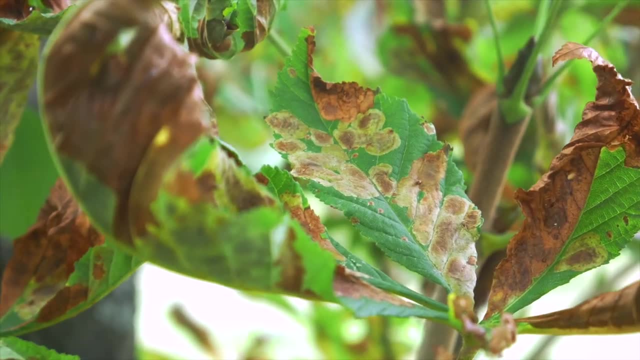 This is an essential skill for the Soil Food Web Consultant to have, as making biological compost is how we multiply our beneficial soil microorganisms and inhibit disease causers. This is achieved by using a close control composting method that Dr Elaine Ingham has. 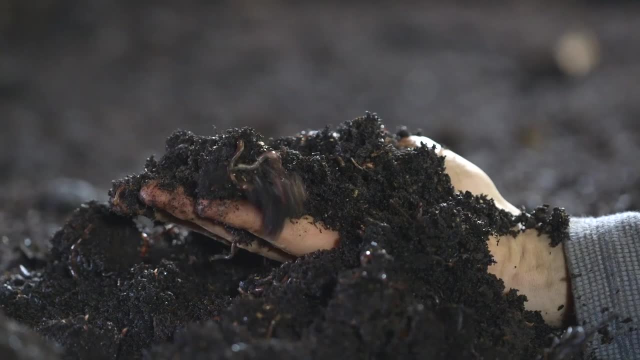 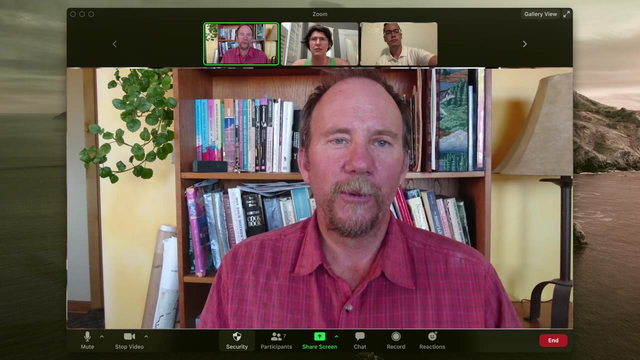 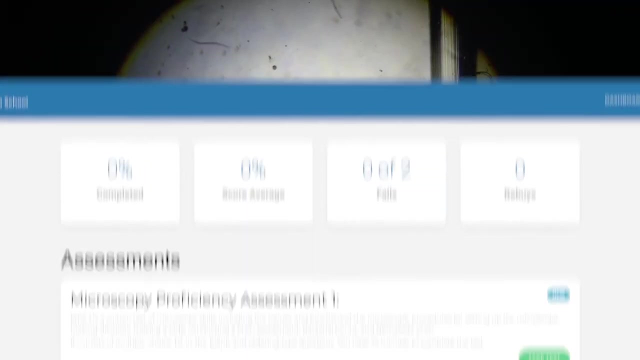 developed over the last four decades. Creating a potent inoculant and then using it to treat the soil is key to rapid soil regeneration. You will also work with your mentor on developing your microscopy skills. At the end of stage 1, you will be certified as a soil food web lab technician. once you have. 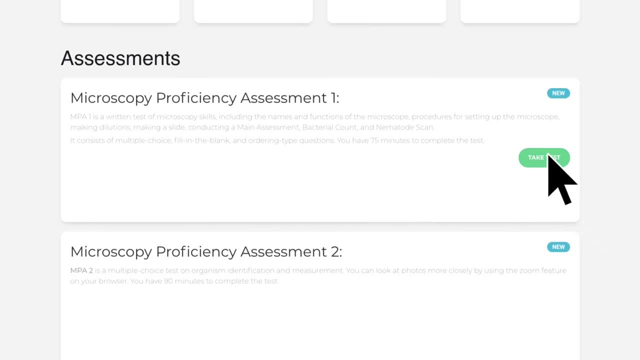 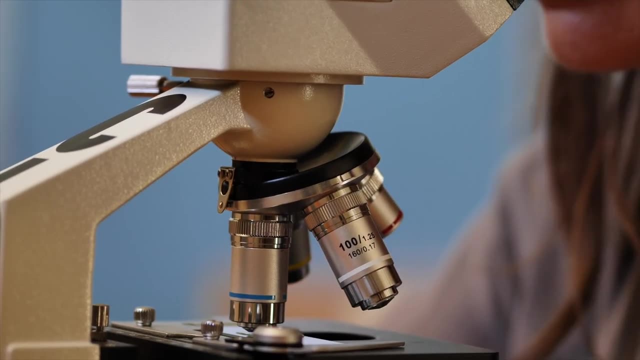 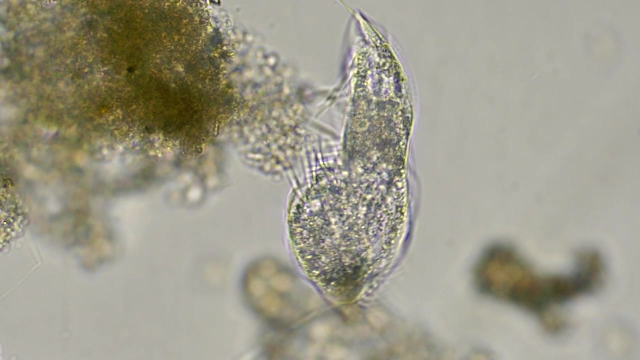 successfully completed the microscopy proficiency assessment. The microscope is an invaluable tool that will give you the ability to assess the quality of compost and liquid amendments before your clients invest all the time and effort that's required in applying them to their land. The microscope is also used to monitor the progress of the microbial community in 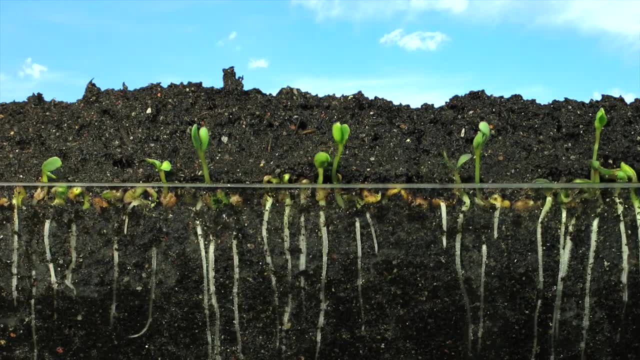 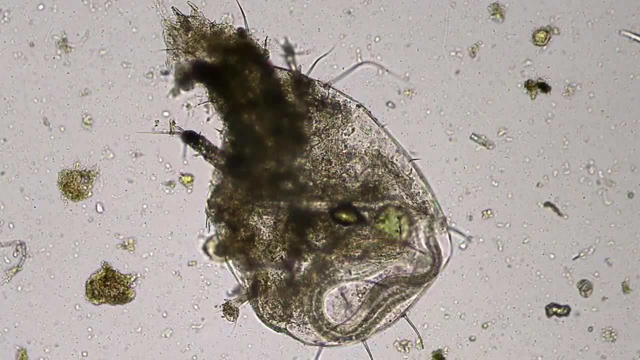 the soil over time so you can take remedial action if required. Farmers you work with will appreciate being able to really see what's going on in their soils at a microscopic level for the first time, and conducting soil assessments will be a significant part of your job. 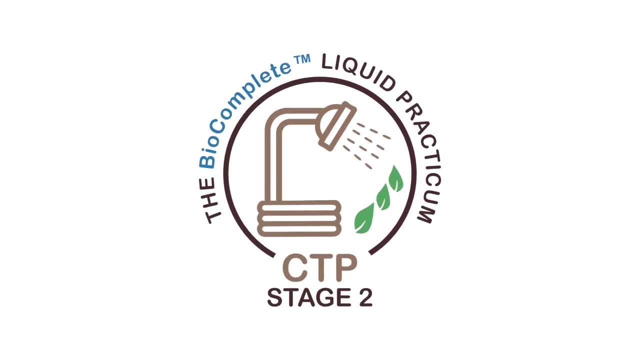 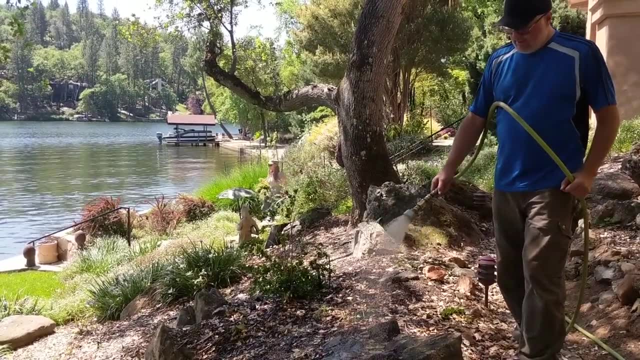 In stage two, you'll use your compost to make liquid biological amendments, which are used for foliar applications or soil drenches. This is a fast and effective way to inoculate your soil with the plethora of beneficial soil microbes that are required to accelerate your soil regeneration. 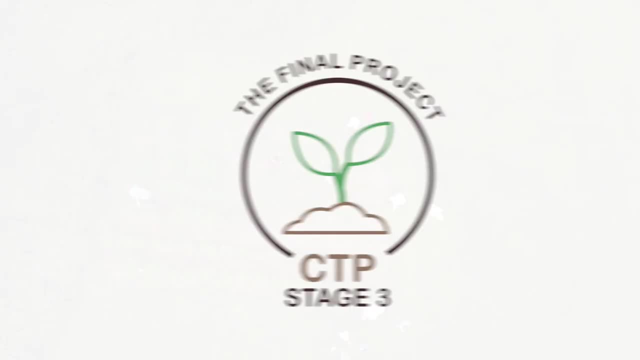 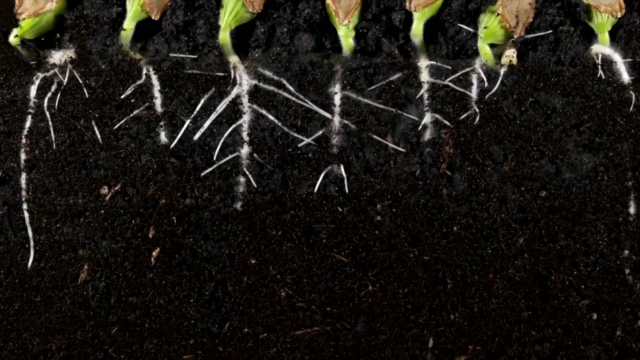 And in stage three, you will be using your amendments to regenerate a small patch of land in the final project. Your mentor will be there to guide you through the process of applying the amendments you created to the soil and the foliage of your plants. You'll use the microscope and other tools to monitor the changes that will start to 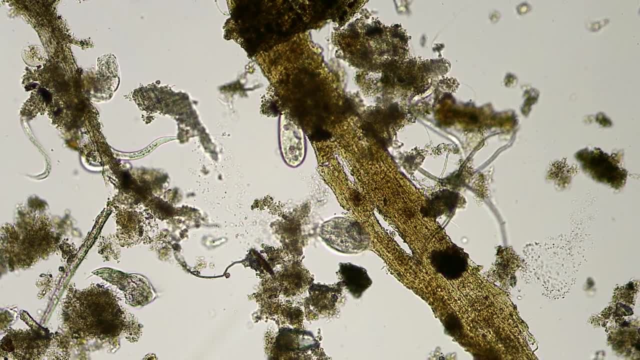 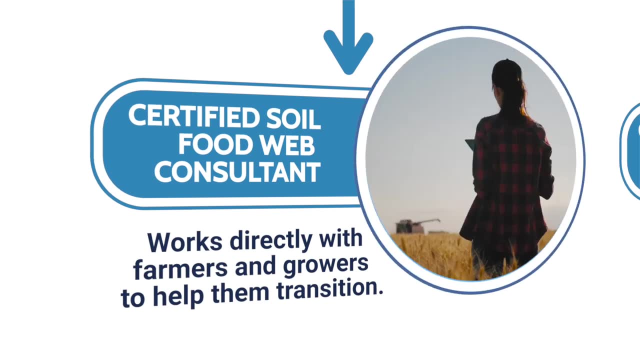 happen as your soil begins to function as a vigorous ecosystem. At the end of the three stages, you will be certified as a Soil Food Web Consultant so you can start working with farmers to help them transition away from chemicals to working in harmony with nature. 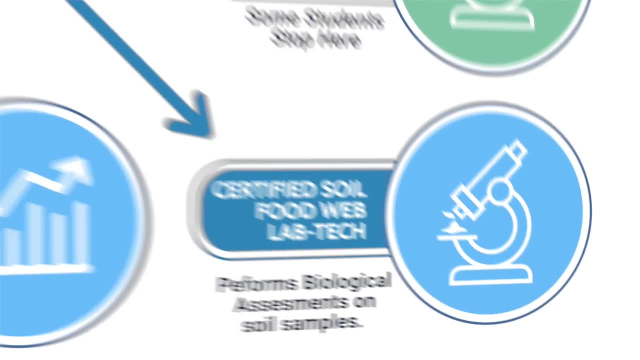 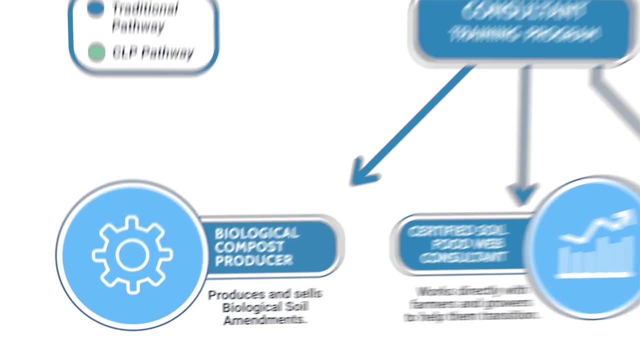 You will also be certified as a Soil Food Web Lab Technician, Which qualifies you as a Soil Food Web Lab Technician, Which qualifies you to perform sample analysis for local farmers and growers, And you will be qualified to make biologically complete soil amendments, including compost. 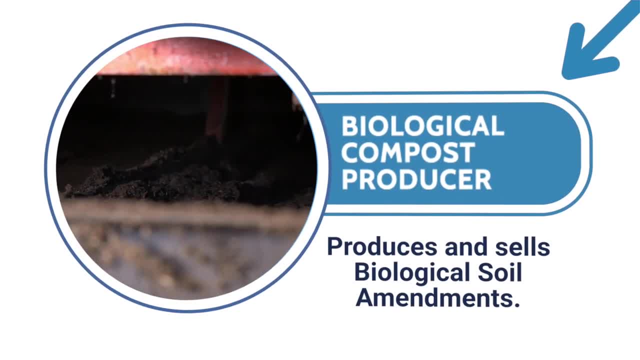 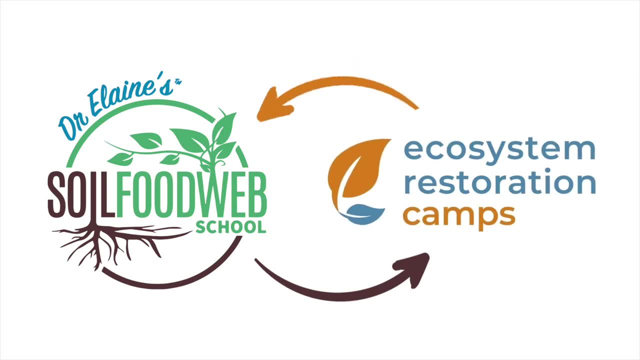 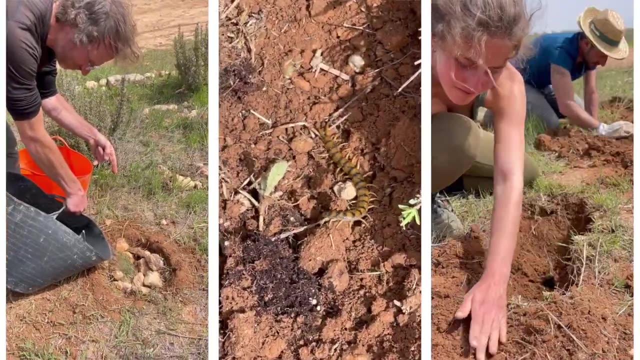 extracts and teas that meet the minimum biological requirements for soil regeneration. The Soil Food Web School is proud to be collaborating with Ecosystem Restoration Camps, a global movement that is on a mission to train people to restore degraded ecosystems around the world. Together, we are developing a series of exciting 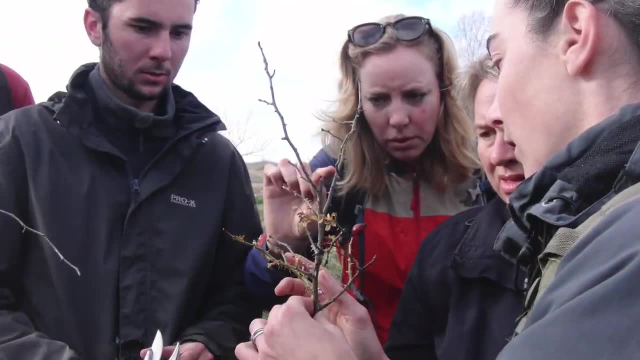 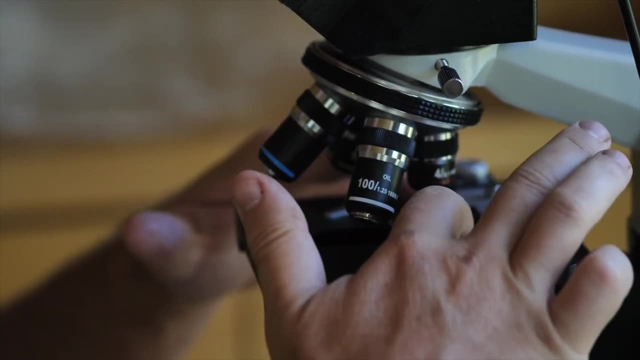 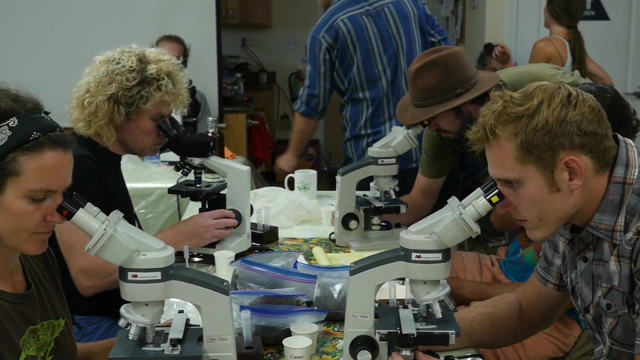 new training programs designed to make it possible for individuals with no previous experience to work together on restoring their ecosystems. These programs will also empower Soil Food Web Consultants to make a bigger impact on the wider ecosystem when they work with farmers who are making the transition to regenerative. 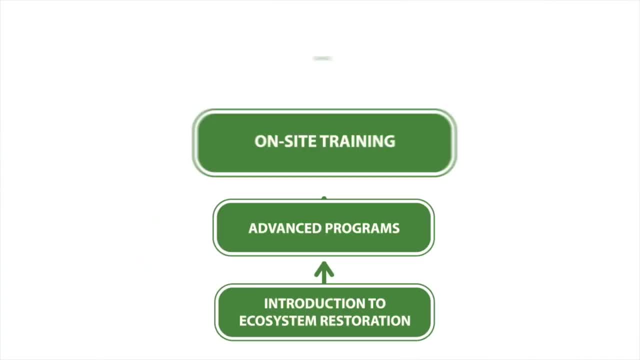 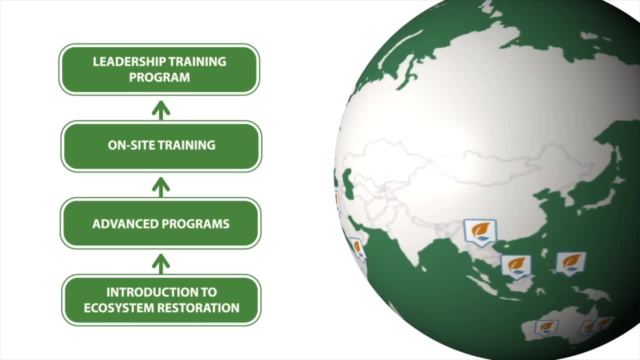 agriculture. There will be beginner, intermediate and leadership level training, both online and at Ecosystem Restoration Camps located in nearly 30 countries around the world. You'll be able to learn more about soil restoration in the next few weeks. You'll be able to develop your skills and experience over time, empowering you to make. 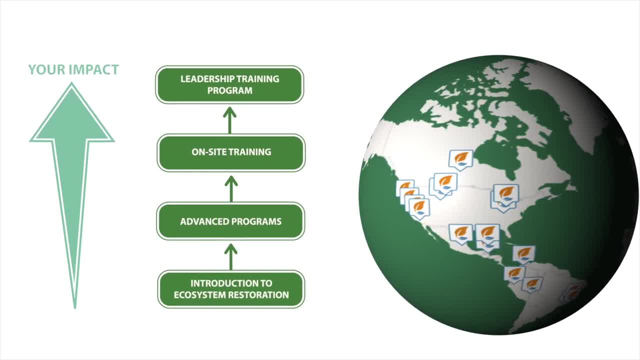 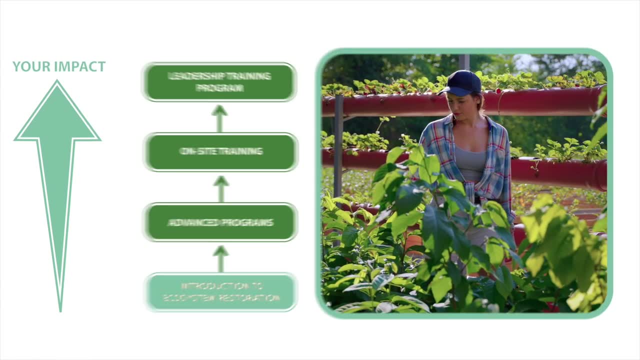 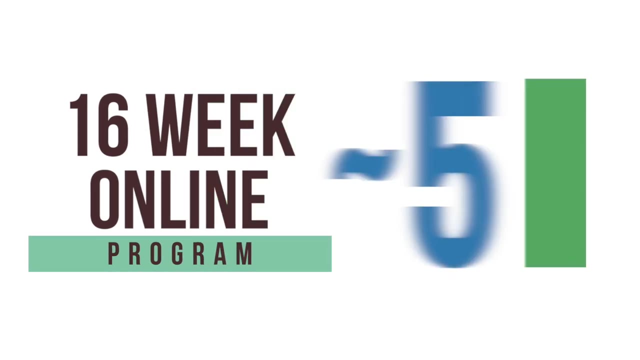 a greater and more valuable contribution as you progress. The first of these programs is the Introduction to Ecosystem Restoration, which covers the principles of ecology and ecosystem restoration. This is a 16-week online program that will require around 5 hours of study per week. 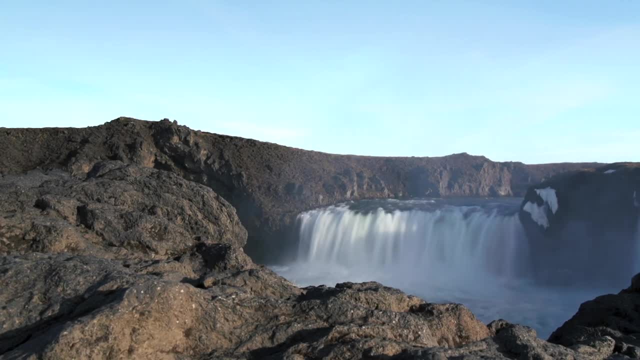 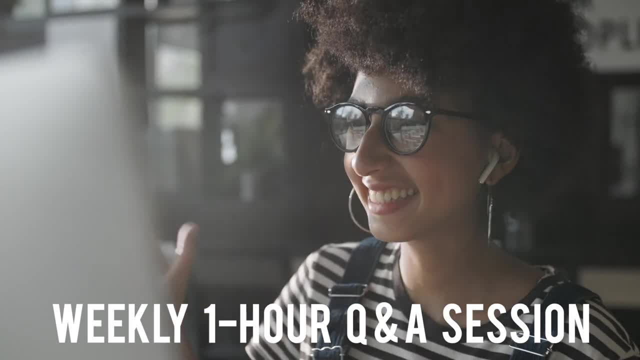 You'll be able to learn more about soil restoration and how they can be used to restore the environment. You'll have a weekly one-hour question and answer session with Paul Morris. You'll also have access to a dedicated forum where you can interact with other students. 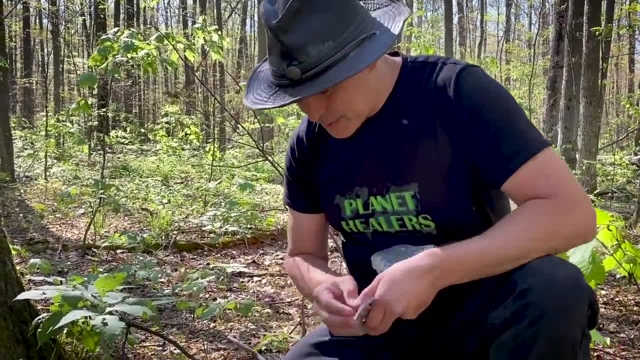 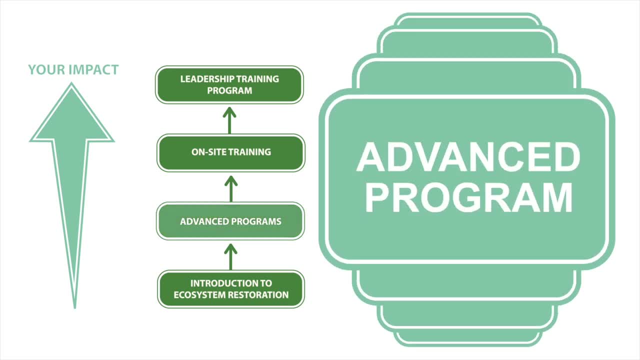 and ask any additional questions. that will be answered by Paul and the team. Once you have completed the Introduction to Ecosystem Restoration, you'll be able to take one or more of the advanced programs, which are each specific to a different type of ecosystem. 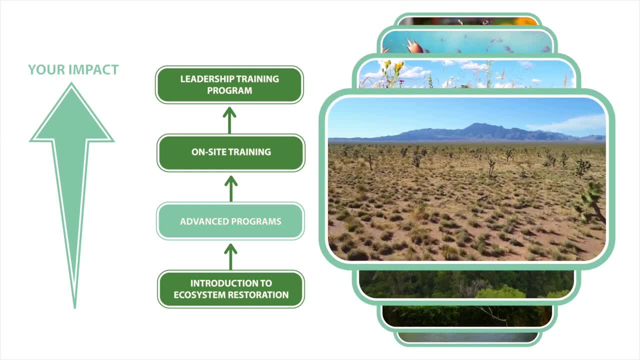 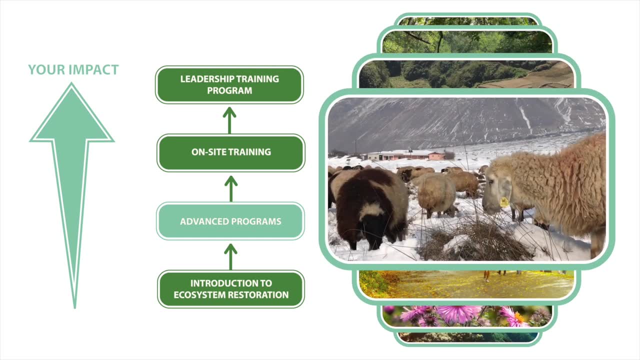 such as tropical rainforest, deserts and dryland, meadows and grasslands, coral reefs, gardens and more. These programs will become available online over the next few months. These programs will become available online over the next few months. These programs will become available online over the next few months. 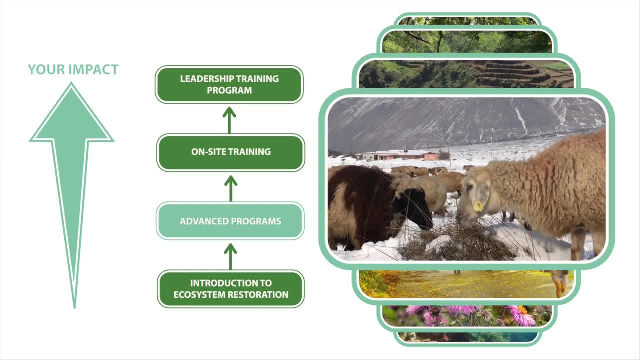